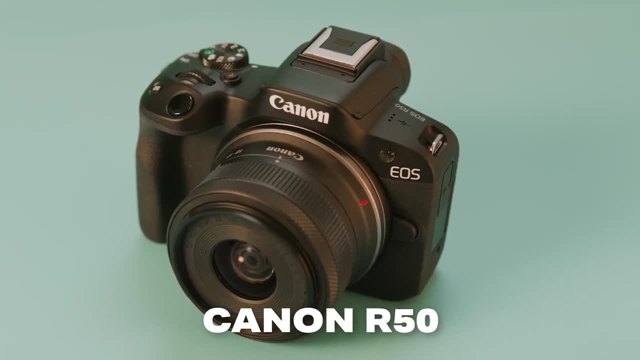 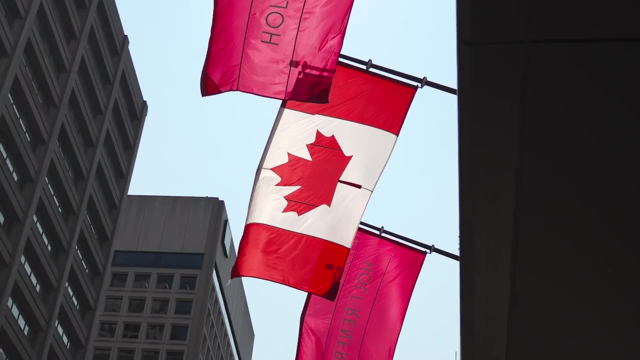 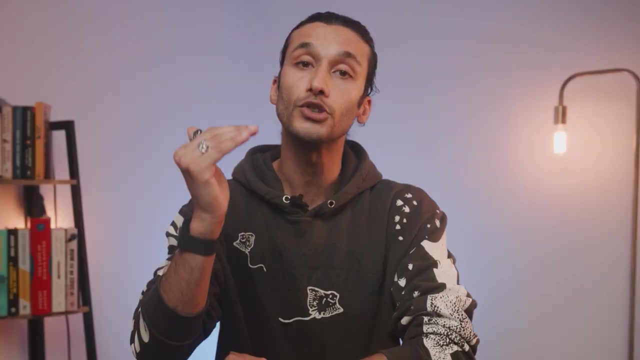 you need in a good camera, And that is the Canon R50.. The R50 has a 24 megapixel APS-C size sensor, which is the sweet spot for resolution and sensor size, In my opinion. it gives you plenty of detail to crop in and zoom into your image, but by having a smaller APS-C size sensor, you also manage to. 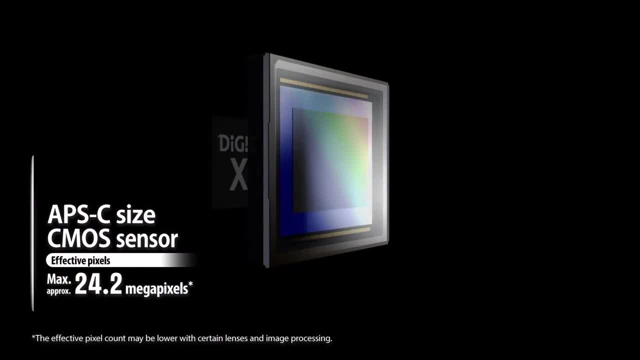 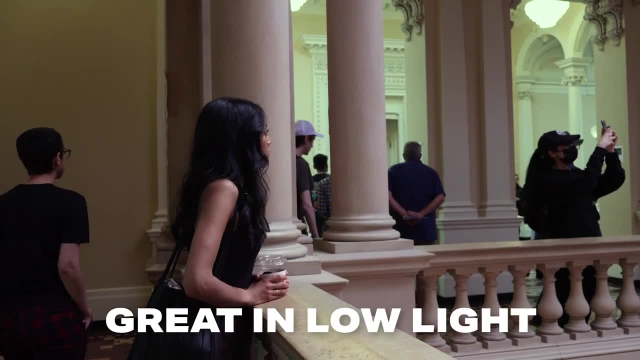 keep your cost for your camera much lower, And it also has an updated processor that gives you a whole bunch of new features that you can use to make your camera look better. So if you're normally see in a budget camera including really good low light performance and an incredible AI, 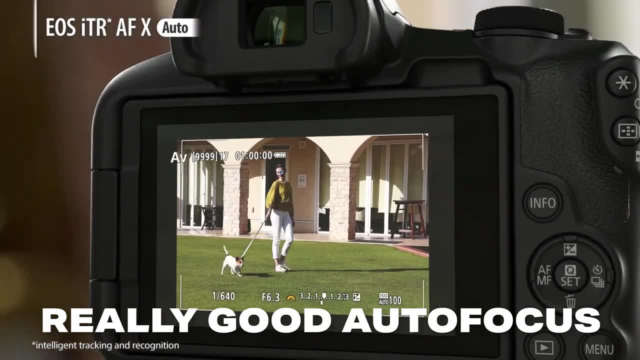 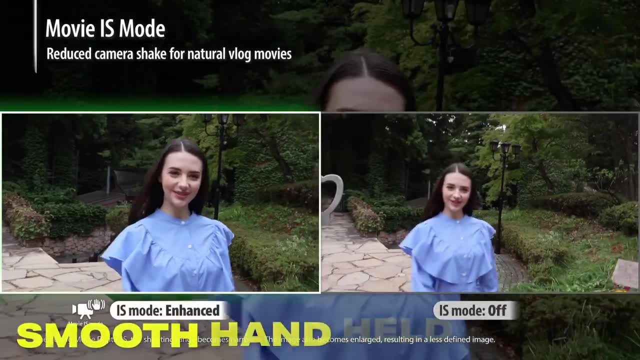 based autofocusing system that does a tremendous job at tracking subjects, because it can intelligently recognize if it's looking at people, animals or vehicles. Plus, it also has digital stabilization for ultra smooth handheld video, and it can shoot photos at a ridiculous speed of 15 to. 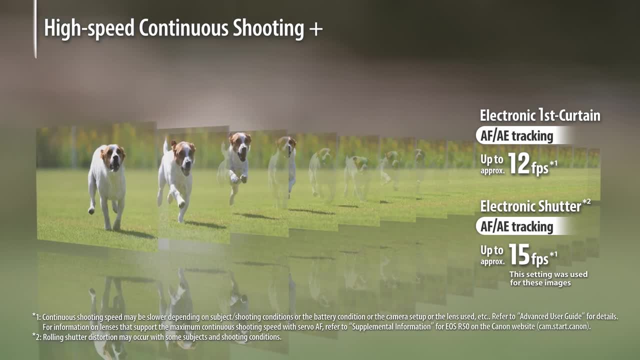 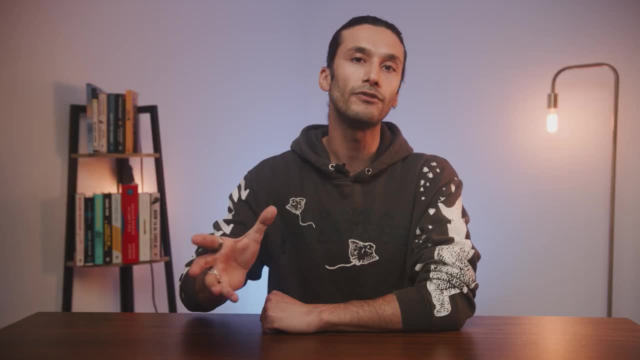 12 frames per second, which is fast enough for any kind of fast moving action, And it can take photos between 28 to 42 JPEGs in a row, And it can also take photos before this camera needs a break, which is plenty of photos, if you're. 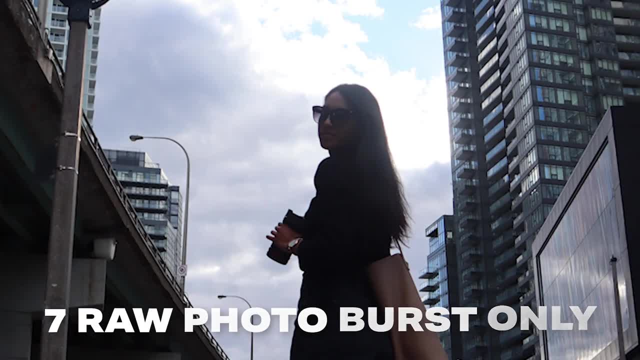 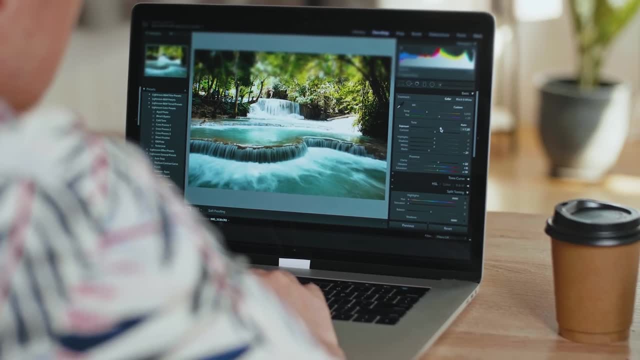 shooting action. However, the one downside is is that it can only shoot seven raw photos in a row. However, you won't really need raw, unless you're planning on doing some heavy editing with your photos, in which case this may not be the right camera for you. And I do have something for you. 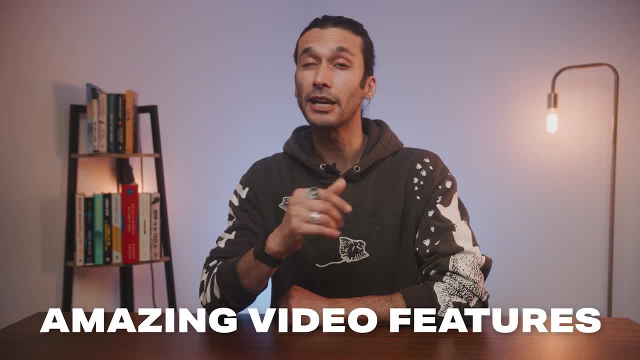 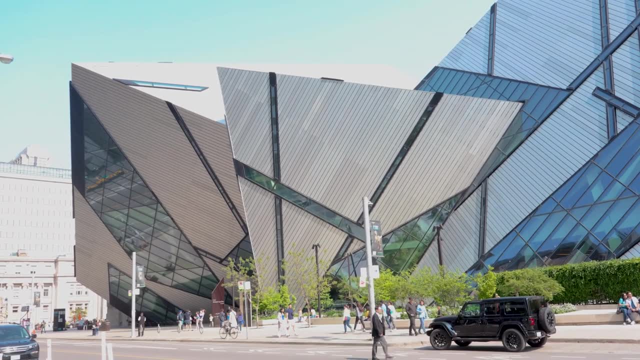 later in this list. But video is where the R50 really impresses me and why I think most people should consider buying this as a budget video camera. It shoots 4K at 24 and 30 frames per second, but that 4K video is actually downsampled from 60 frames per second, which is a lot, So 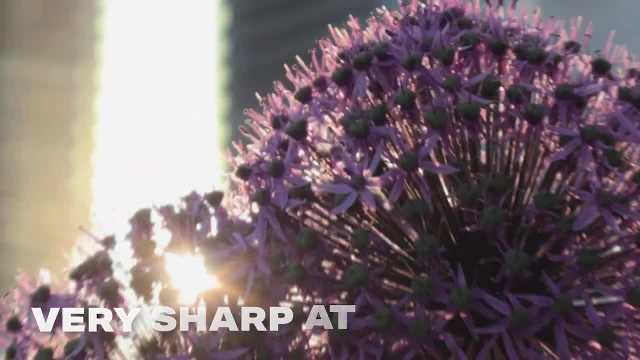 that's why I think it's worth considering buying this as a budget video camera. It shoots 4K at 24 and 30 frames per second, but that 4K video is actually downsampled from 70 to 6K, which means your 4K video really has the detail and clarity of 6K, which is a lot more. 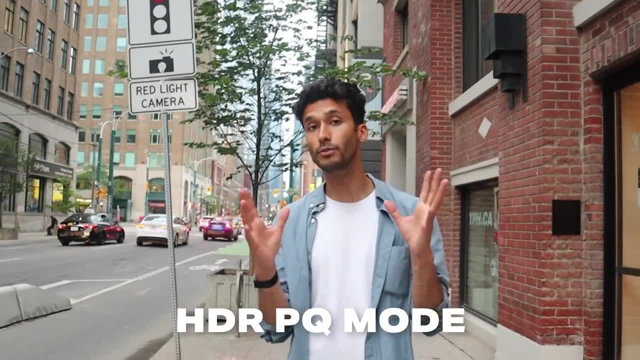 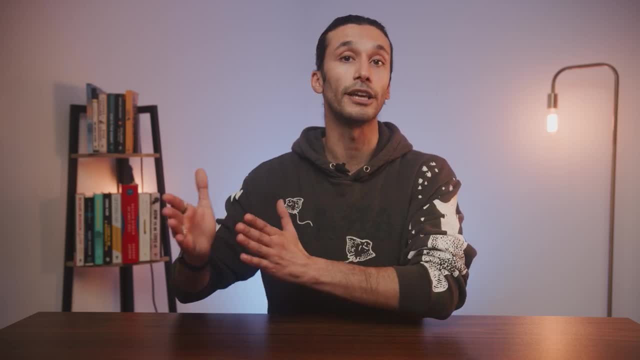 than 4K, And it also lets you shoot in HDRPQ mode, which gives you a little bit more dynamic range, but also 10 bit color, which is perfect for someone that wants to take their video and edit the colors later on. Plus, it has slow motion in full HD at 60 frames per second. 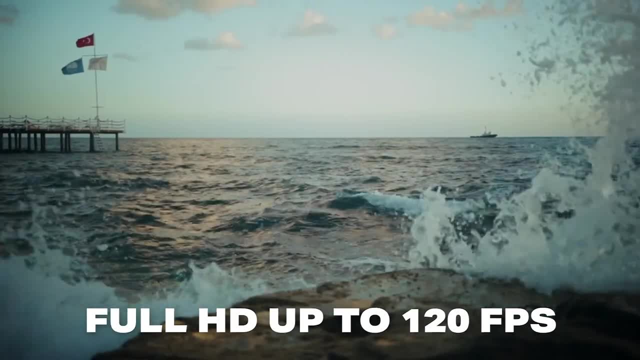 for two times slow motion and 120 frames per second for five times slow motion. Now, design-wise, the R50 is a really small and compact camera. perfect for someone who wants to use it for traveling, or if you're looking for a camera that's easy to use, or if you're looking 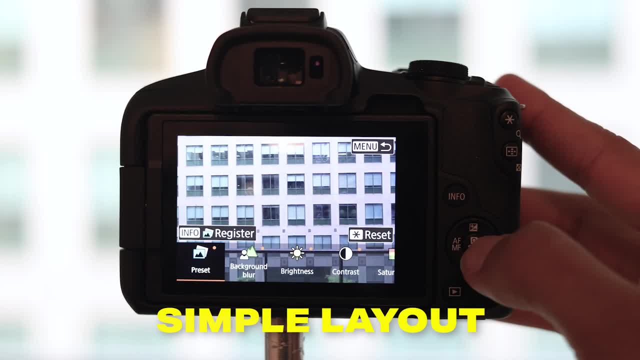 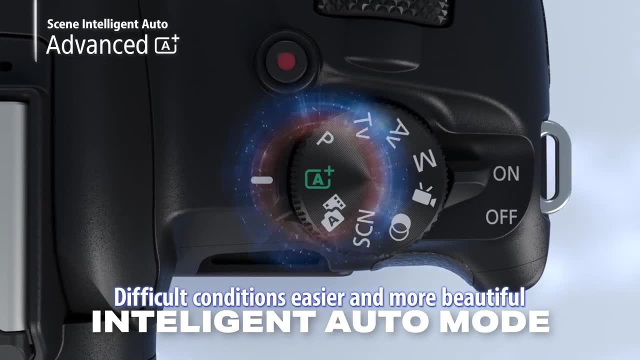 for something that's easy to carry around or just an everyday carry camera. The bun layout and menus are super simple. It's a really easy camera to just pick up and get great results with, And on top of that it also has something known as intelligent auto mode. 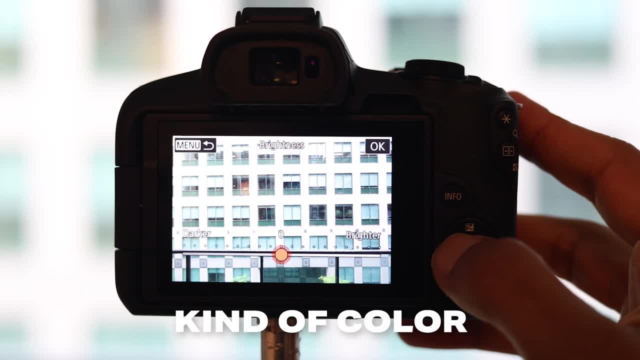 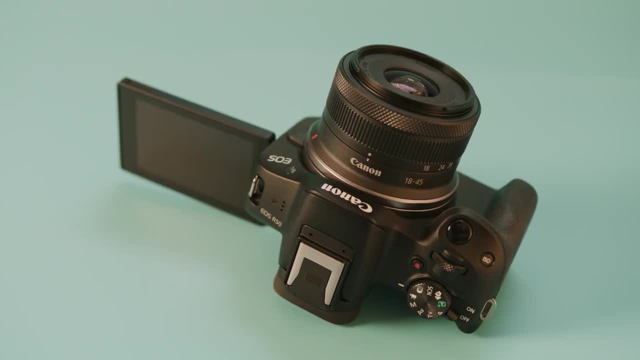 where you tell the camera how much brightness, contrast, what kind of colors you want, and the camera figures out all the complex settings for you, taking all the guesswork out of getting great photos. And the R50 also has a side articulating screen that has touch control. 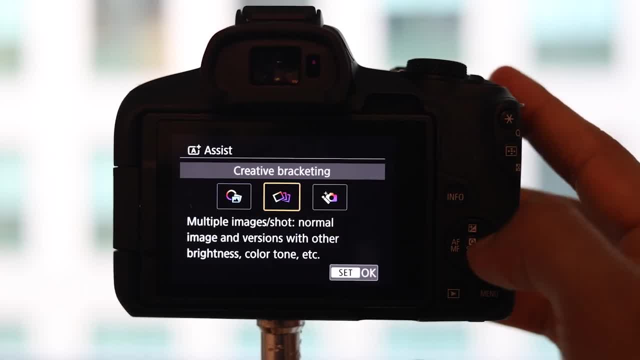 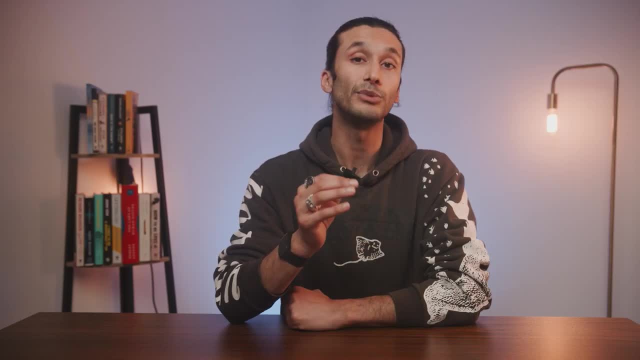 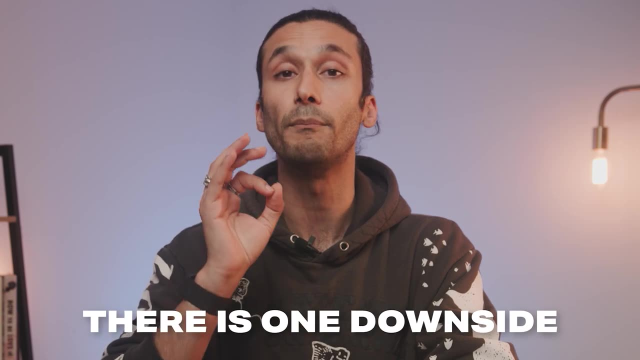 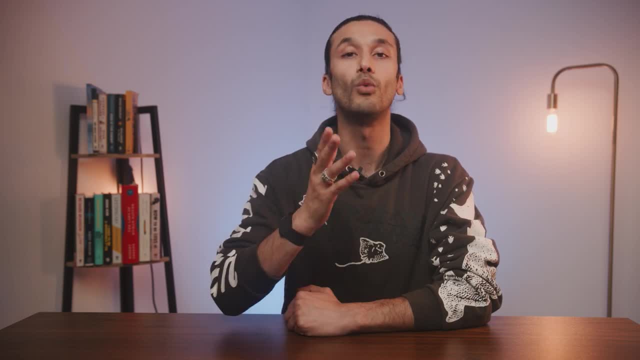 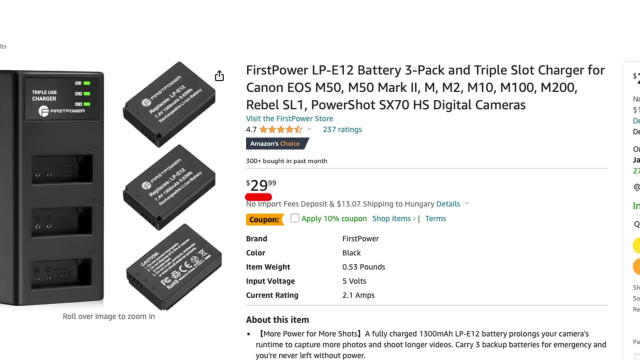 typical for a budget camera, but you will want to make sure you have one or two spare batteries on hand. But if you want spare batteries, it's pretty easy to get a two pack on Amazon for as little as $20 to $30.. The R50 pretty much gives you everything you need at a great price And 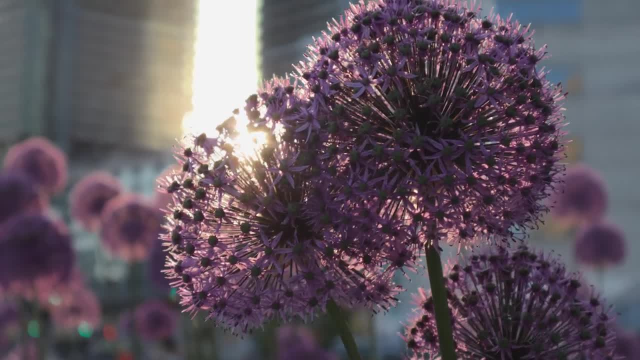 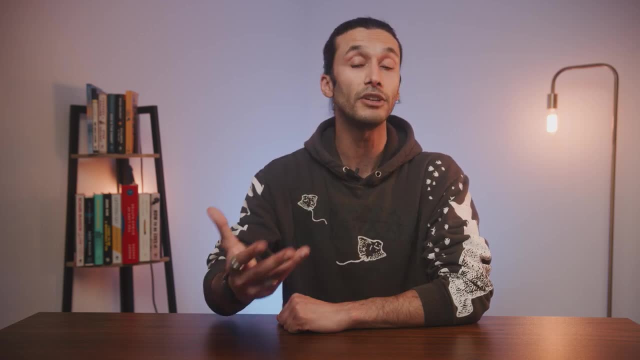 I'm really impressed by how powerful this camera is, And I'm really impressed by how powerful this camera is, considering it's only a beginner and casual camera, And another camera that I really like for beginner and budget shooters who specifically want to vlog and make videos. 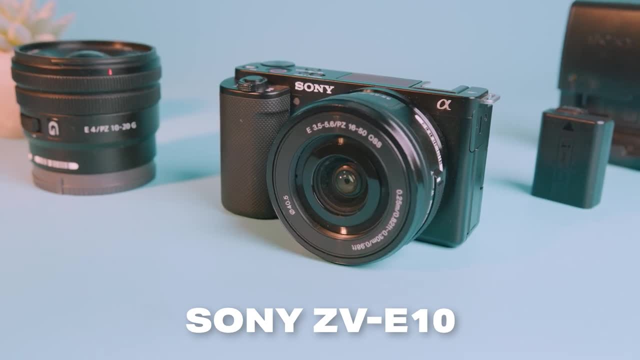 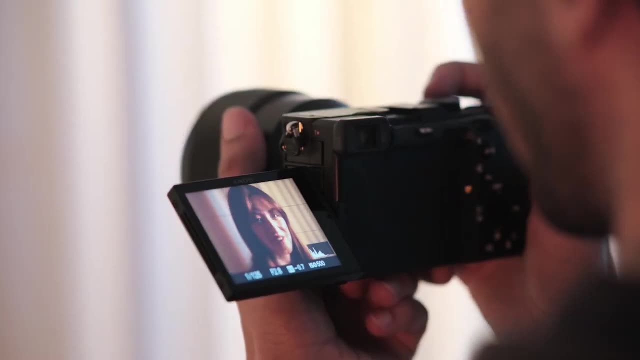 is the Sony ZV-E10. And it does a few things that the Canon R50 does not. The first thing you notice about the Sony ZV-E10 is that it has a really unique body type, And that's because who this camera was designed for. It has a really simple button layout with just one button to switch. 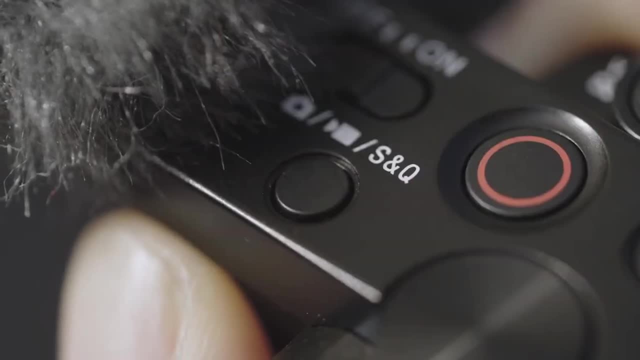 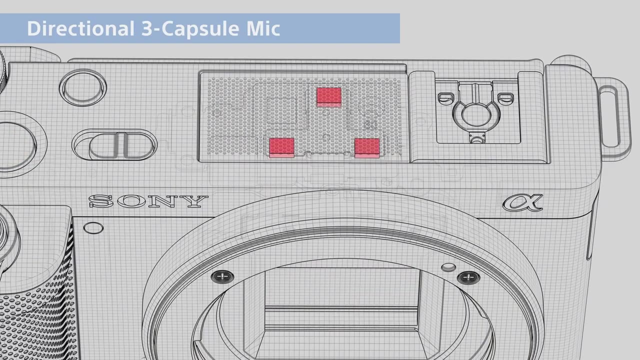 between photos, videos and slow motion, And there's no messy mode dial. With two separate record buttons for photos and slow motion, you can switch between the camera and the R50. And the R50 has a three capsule microphone built right into the camera. that gives you almost the same quality. 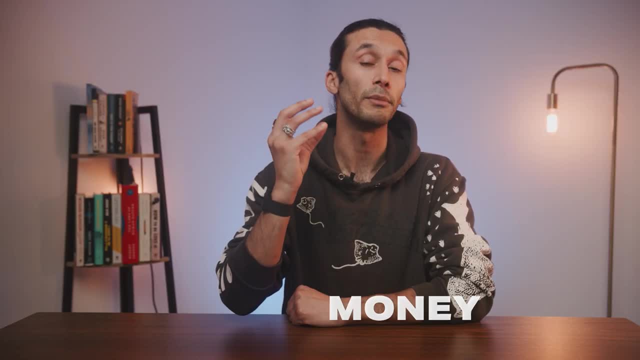 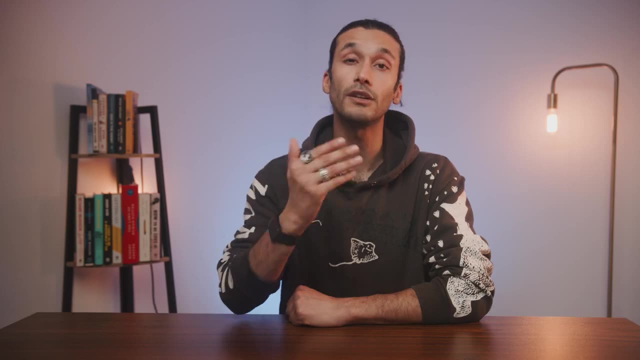 as an external microphone, saving you money and also keeping your camera much smaller if you're planning on vlogging with it. But one thing to know about the Sony ZV-E10 is that it does not have an electronic viewfinder, which some photographers may not like. but the ZV-E10 is. 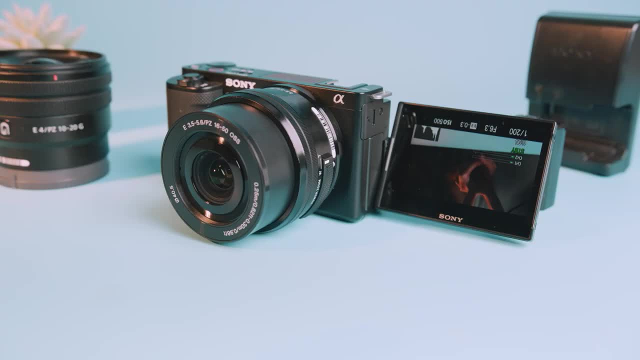 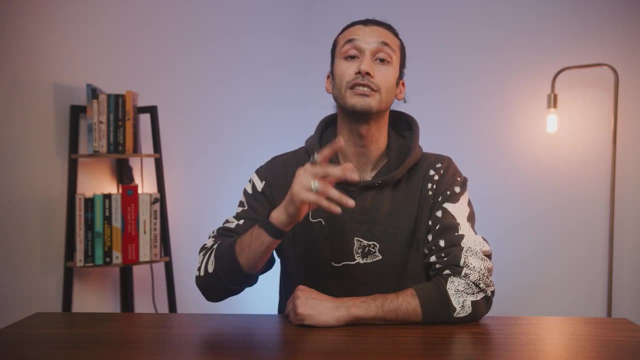 still a very, very good photo camera. It does, however, still have a side articulating screen, while the side articulating screen doesn't have the full touch controls that you see on the Canon R50, but the ZV-E10 still has touch controls And that's because the ZV-E10 is a very, very good 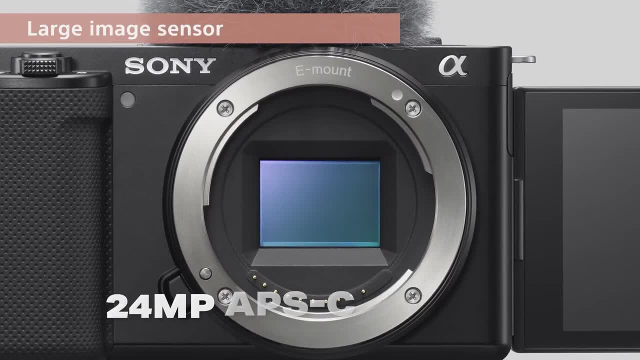 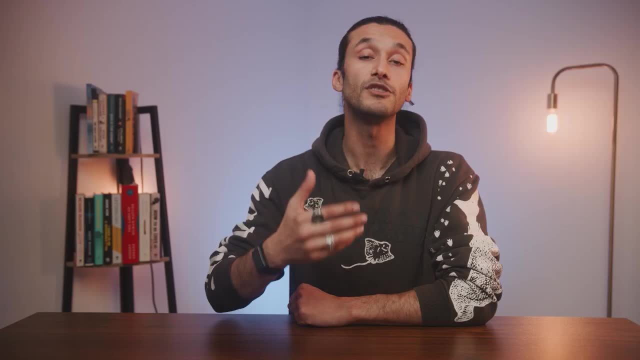 focus. Inside the ZV-E10, you have a pretty standard 24 megapixel APS-C size sensor, which is pretty similar to the Canon R50.. However, because it's a Sony sensor, it does have some additional benefits. For example, it has really good low light performance, even better than the. 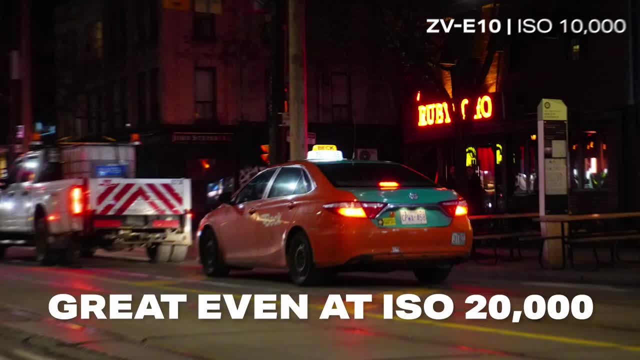 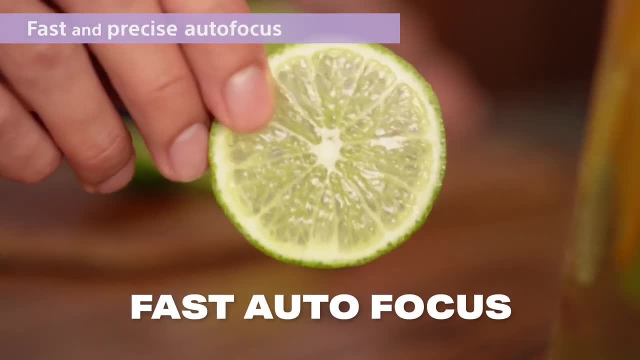 Canon R50, and you can easily shoot as high as 10,000, even 20,000 ISO with very little grain in your photos. And because it's a Sony camera, it also has tremendous autofocus. Now, it's not AI-based autofocus, but the autofocus is ultra reliable and really. 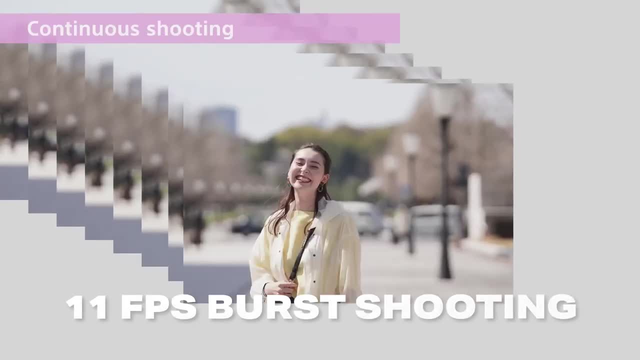 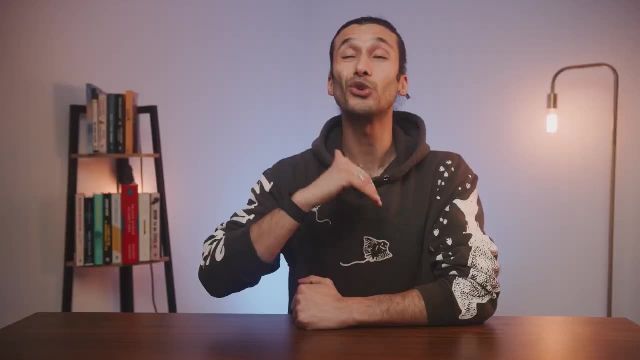 really good at tracking moving subject matter. In terms of photos, it shoots at 11 frames per second, but it can actually shoot 116 JPEGs in a row, or 46 raw photos, which is incredibly impressive, considering the Canon R50 only does seven raw photos in a row. So if you're someone. 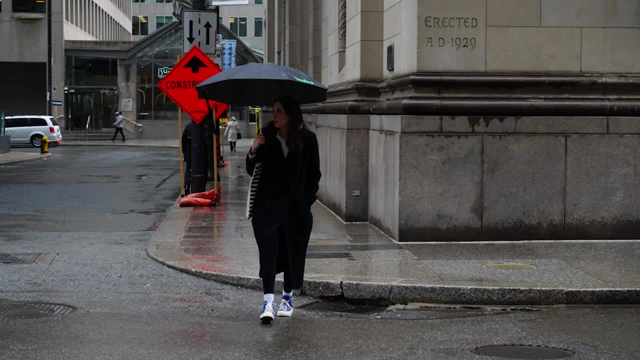 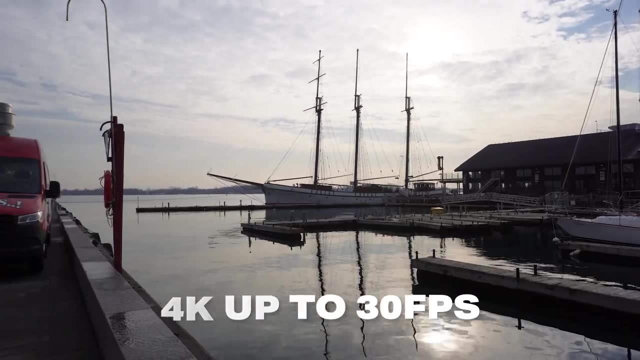 that's planning on shooting a lot of raw photos and heavily editing your images. the ZV-E10 is a much better camera for you than the Canon R50. And video is just as impressive. It shoots 4K at 24 and 30 frames per second, And the video in this camera is also downsampled. 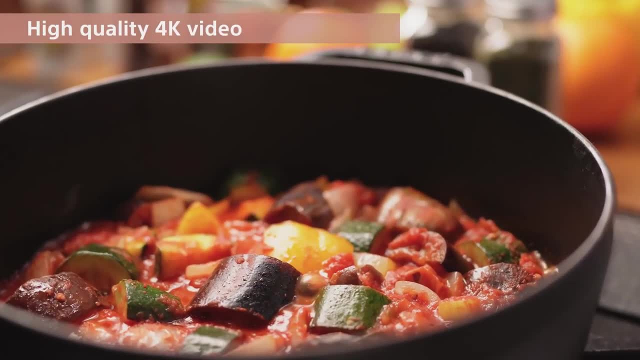 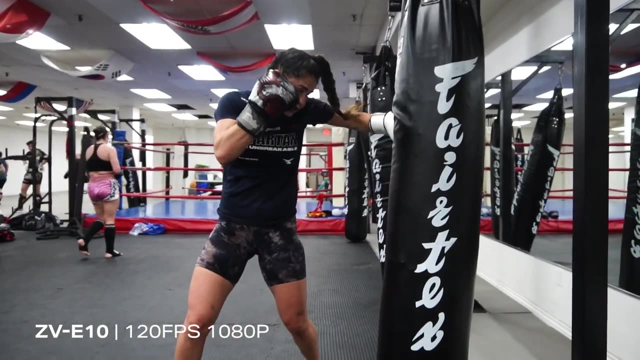 to 6K, So you have 6K clarity in detail in your 4K video. And it also shoots full HD at 60 frames per second for two times slow motion and 120 frames per second for five times slow motion. In terms of video specs, the R50 and the ZV-E10 are pretty much on par. However, there's one thing. 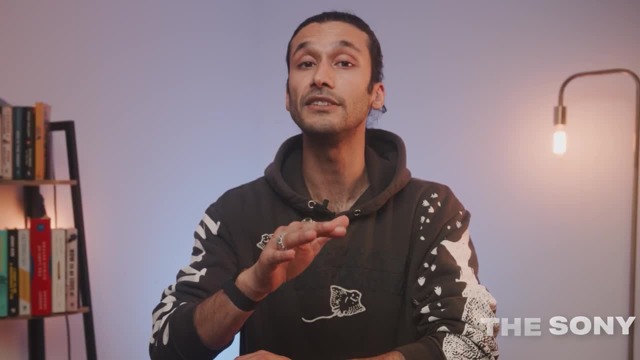 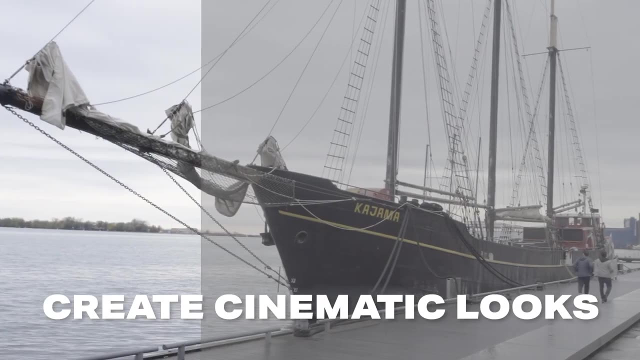 that the ZV-E10 does, that the R50 does not do, and it makes the ZV-E10 a much, much better camera. The ZV-E10 also has long profiles built into it, So if you're someone that really wants to create, 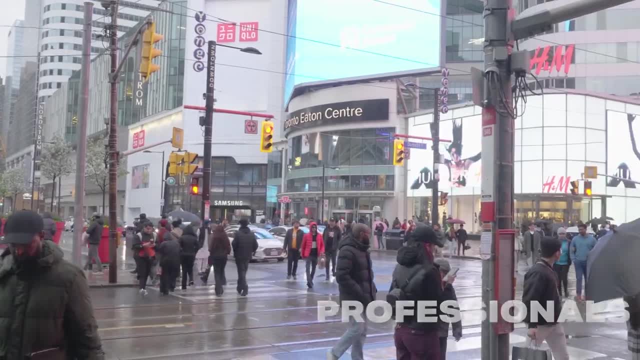 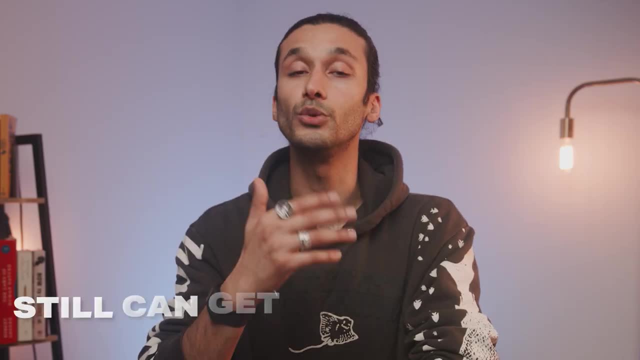 a cinematic look and really do some serious color grading with your video. the ZV-E10 is a much better fit, But one thing to note is that the ZV-E10 only has 8-bit color, but if you know how to grade you can still get a great image from. 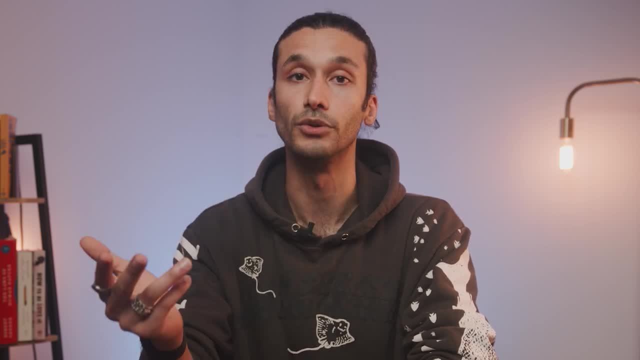 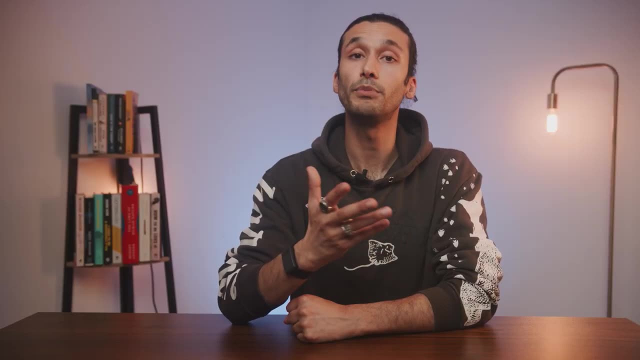 this camera and standard video from the ZV-E10, in my opinion looks beautiful And it also has digital stabilization in camera So you can get really smooth handheld video and vlogs. But once again it does have pretty small batteries. but it's pretty easy to pick up a spare set on Amazon. 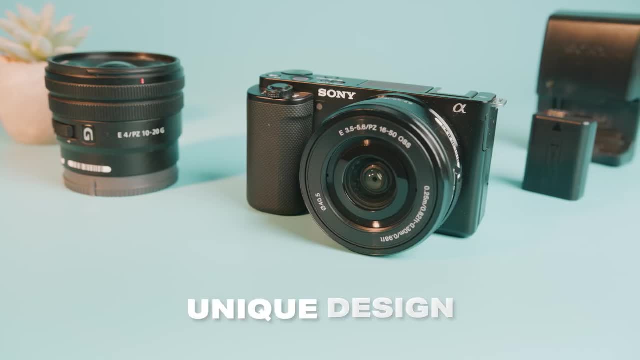 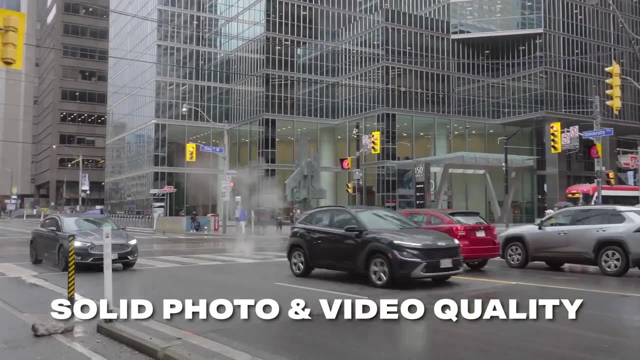 for only 20 to $30.. The ZV-E10 has a really unique design That's going to make it much easier to create online content, especially for vloggers, And the photo and video quality is really solid. The ZV-E10 is a camera that I recommend everyone look at if you're thinking of buying a budget. 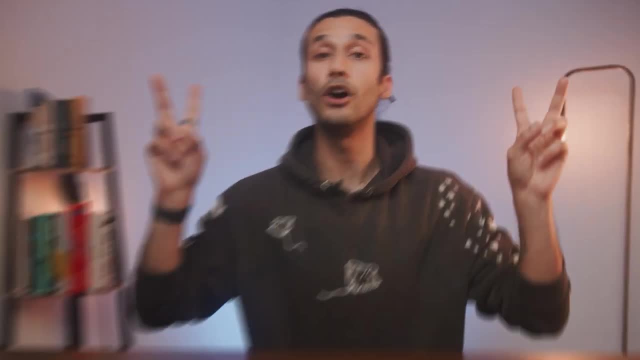 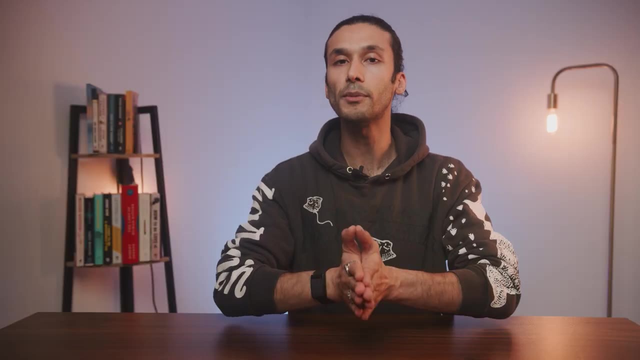 camera for both photos and video. Now, some of you guys might be on an ultra budget. You want a simple camera that's going to take great looking photos with pretty decent video quality, And you probably just want to replace your cell phone or an older, cheap camera you have For you guys. 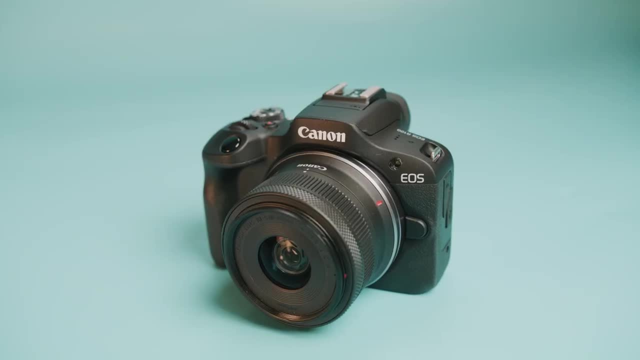 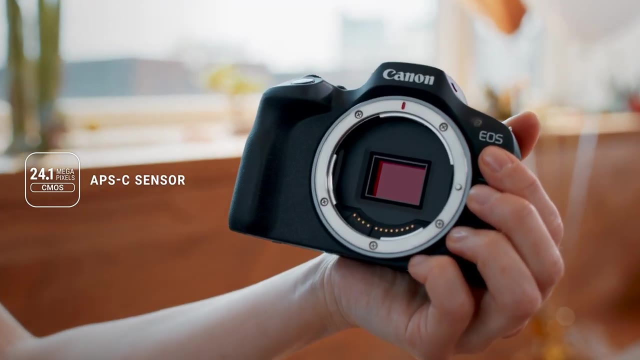 I have the camera that I think does this the best right now, And that is the Canon R100.. It has a 24 megapixel APS-C size sensor, which is pretty much the same sensor in the Canon R50, but with a different processor. It still has really decent autofocus, although without the 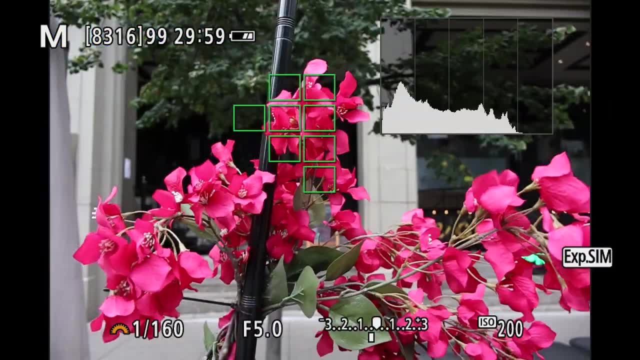 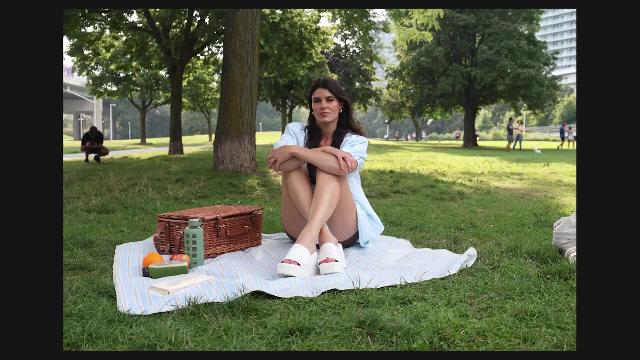 fancy AI tracking In photo mode. this autofocus performs really reliably and it still does a really good job at tracking moving subjects. And in terms of photo and video quality, it's still pretty much the same thing, with a few minor differences that I'll explain. 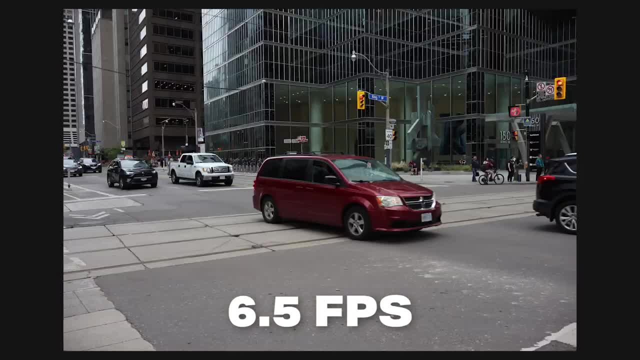 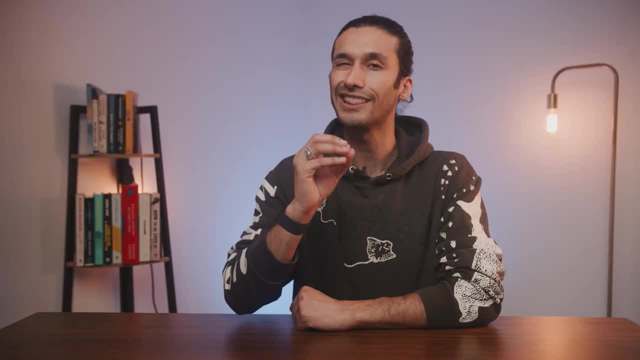 The Canon R100 can shoot photos at 6.5 frames per second, which is an ideal speed for someone who's a casual shooter, just taking everyday photos- or maybe you're on vacation and you just want a lifestyle camera. However, one really cool thing about the R100 is that it can actually take a. 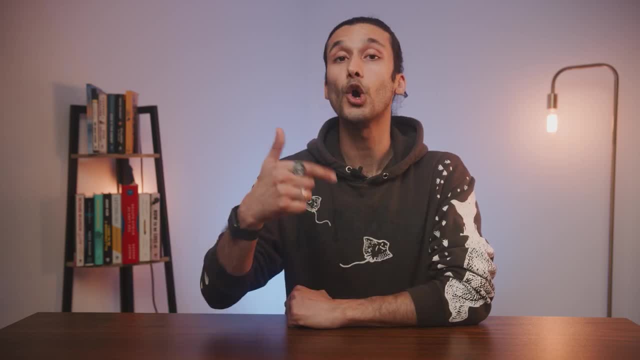 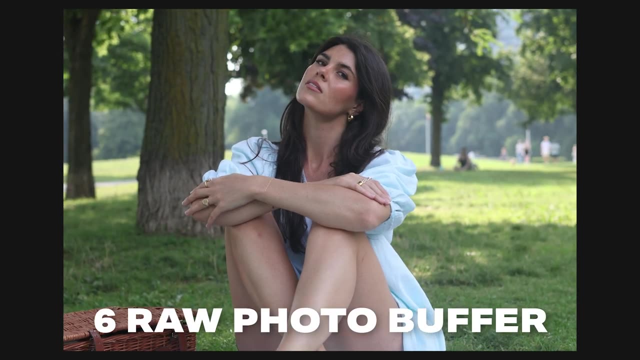 thousand JPEGs in a row, So you can shoot for a really long time and then go back in later and pick the exact shot you want. And it can also take up to six raw photos in a row, which is pretty much the same as the much more expensive Canon R50.. Video wise, the Canon R100 shoots 4K video. 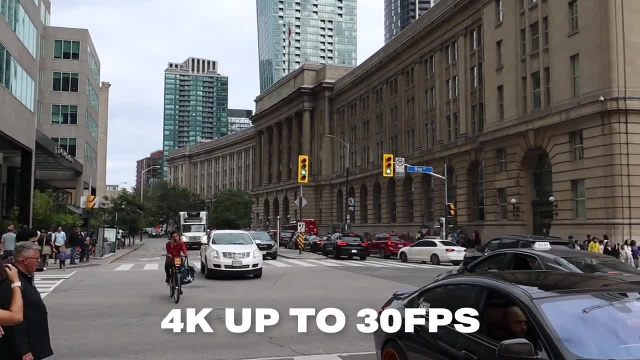 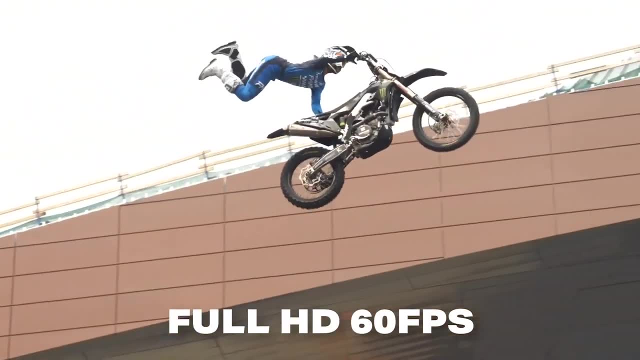 at 24 and 30 frames per second. However, this is regular standard 4K video, not downsampled from 6K like the Canon R50 does, And it also shoots full HD at 60 frames per second and 120 frames per second. And, let's be honest, slow motion looks awesome And you always 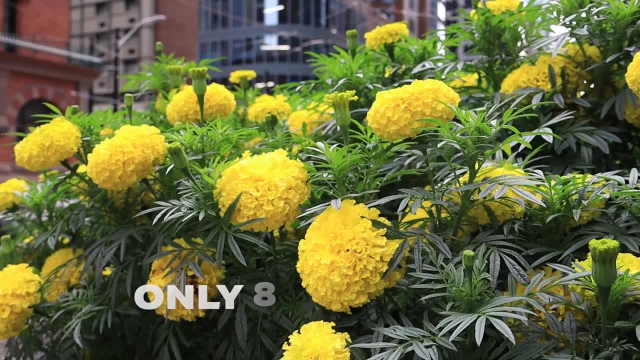 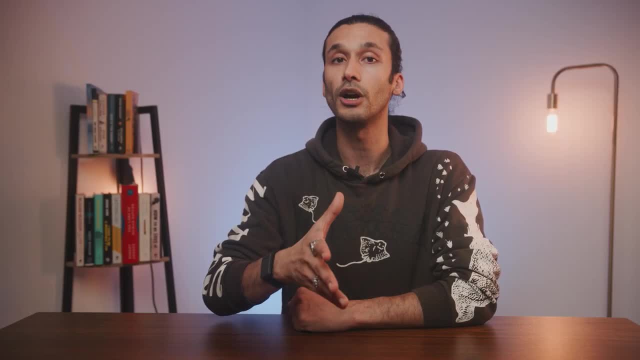 always, always want slow motion in a casual camera, But the Canon R100 only shoots in 8 bit color, which should be just fine for casual users, because you guys are probably not planning on editing your video colors anyways. But the reason I love the Canon R100 as a budget camera: